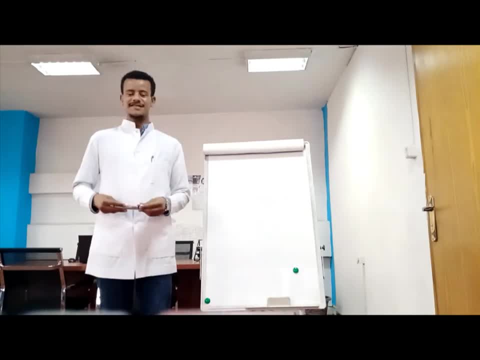 Hello, welcome to our new tutorial. my name is Bela Echandeni. In this new tutorial we are going to talk about the basic procedures of highway design. All of these design procedures are applied with software. Currently, we are working on a new software called Civil Street. 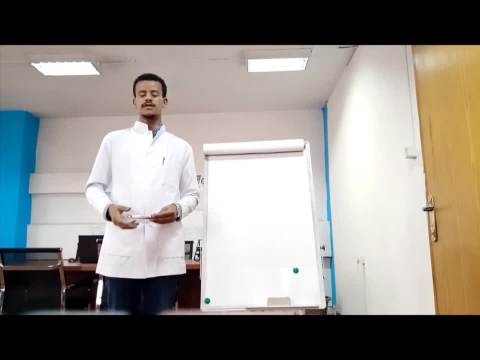 We have completed the design of the road and the road is now ready to be used. We are going to use a new road. it is the Himex road. We are going to use the road that we have to use for the data import and the reportage. 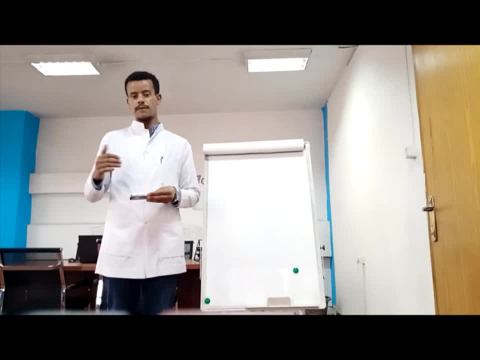 And we are going to use the same route to operate the design of the road. But first we need to make sure that the software is working properly. Then we have to start the process of internalizing the software. I would like to share with you the same software solution that we have been working on for a long time. 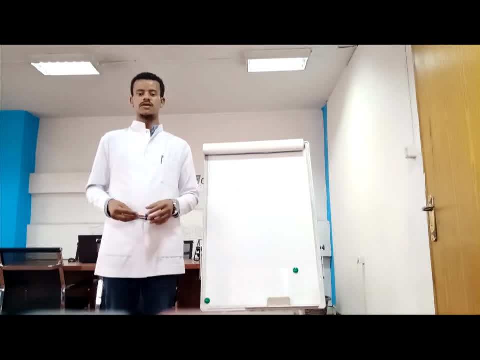 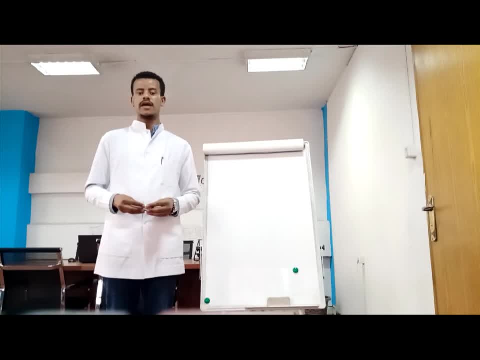 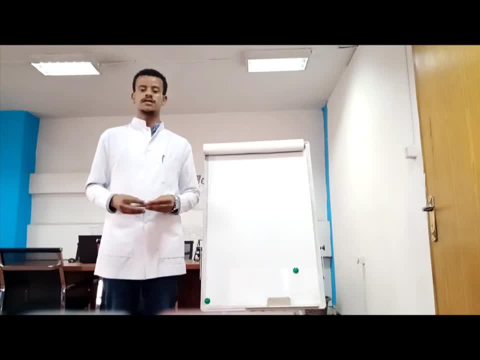 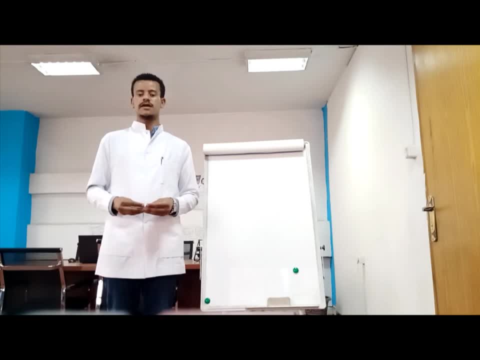 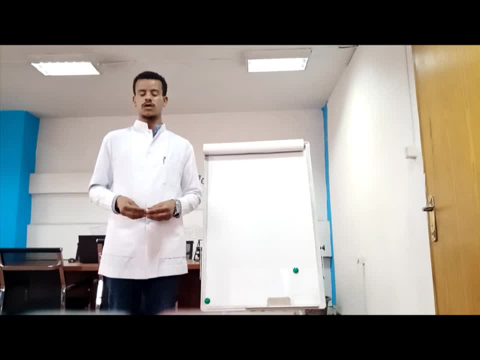 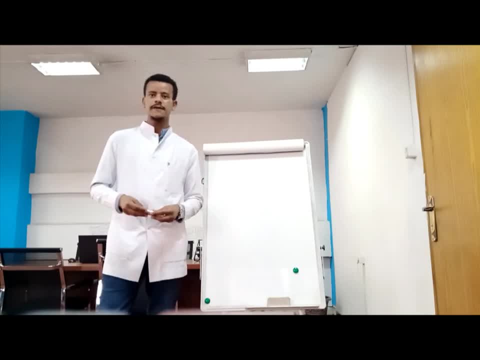 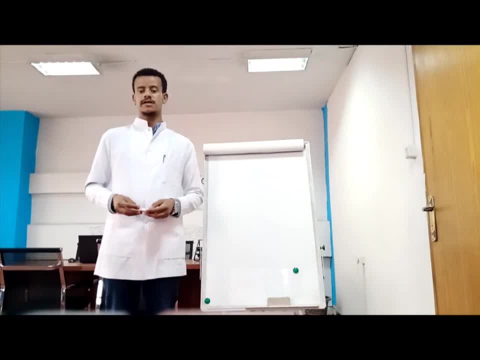 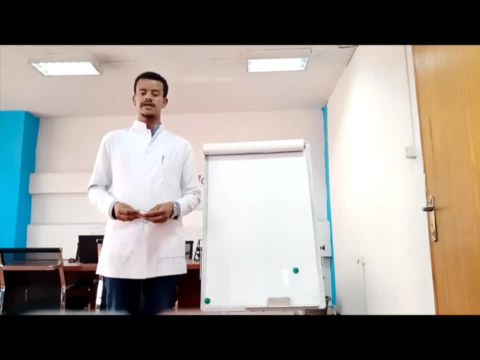 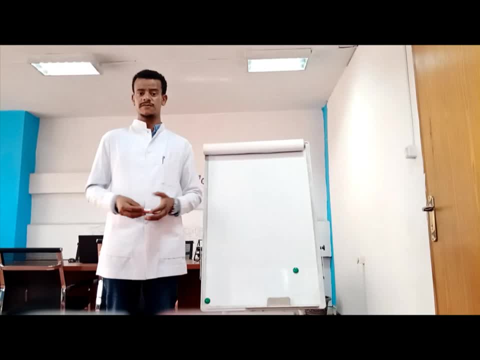 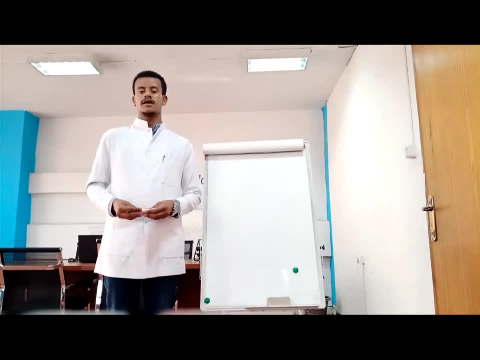 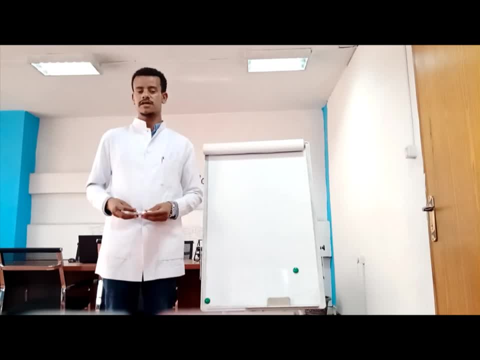 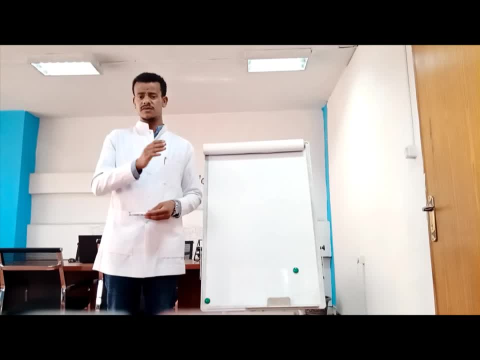 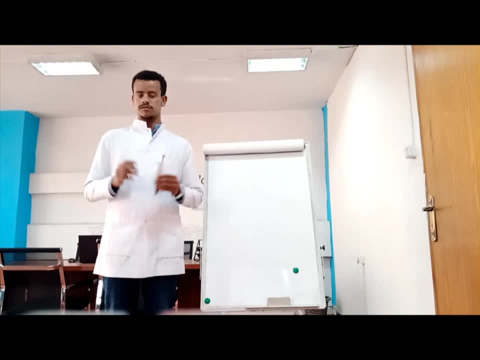 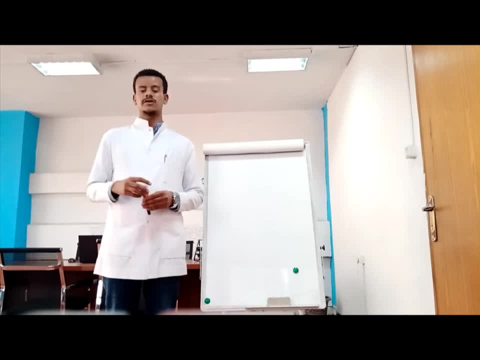 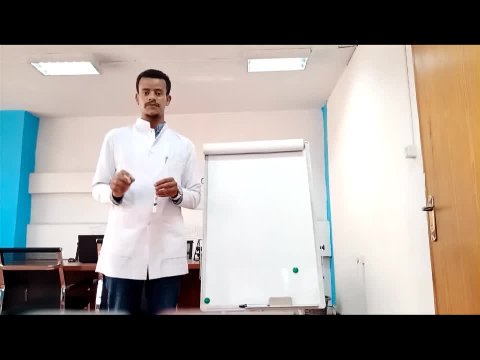 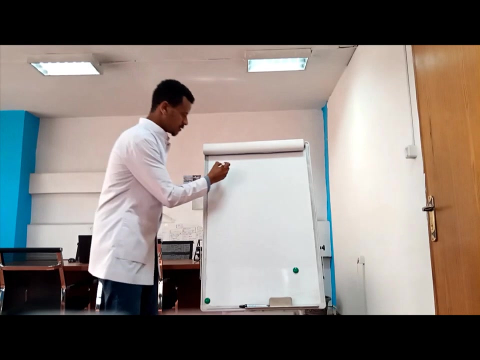 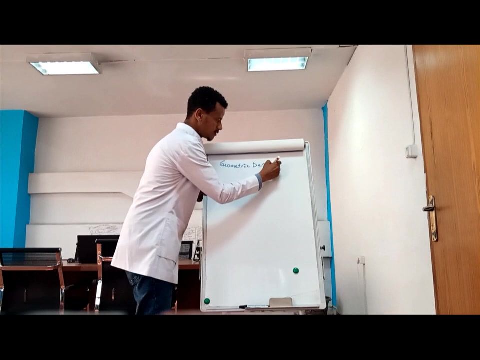 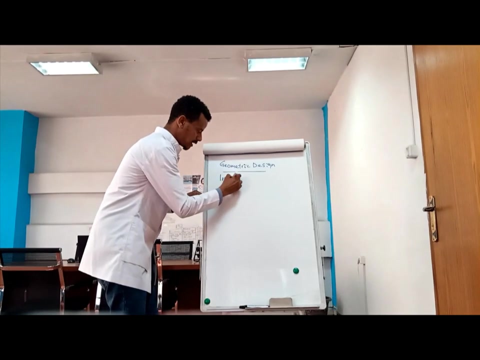 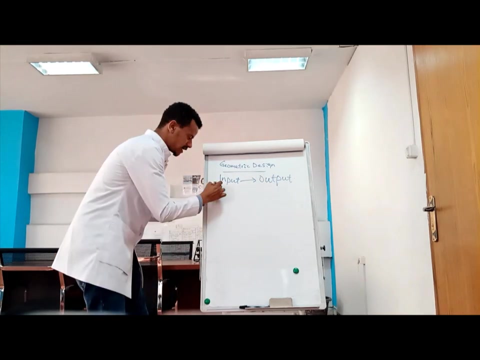 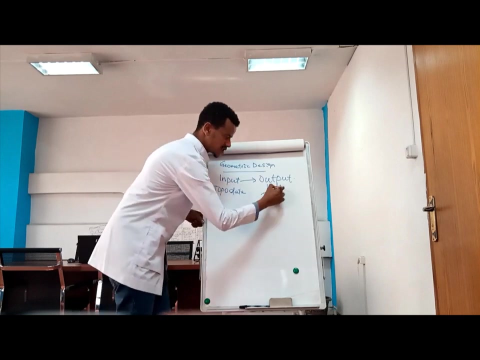 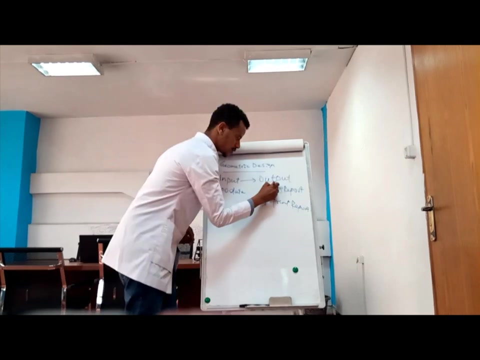 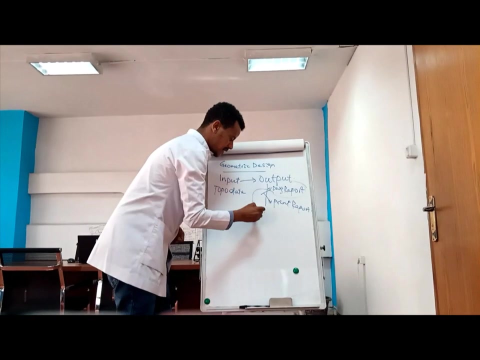 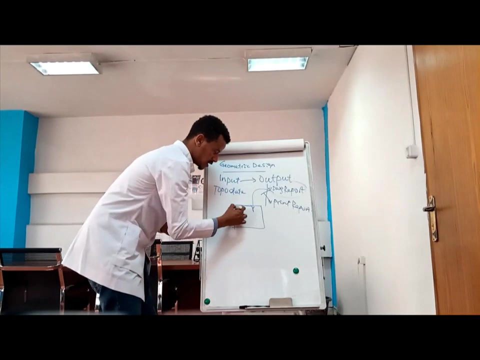 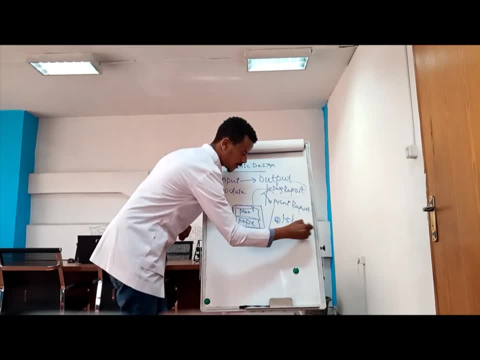 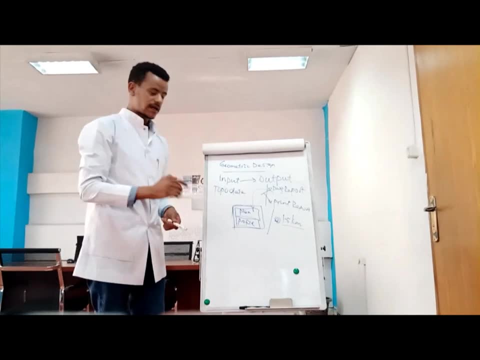 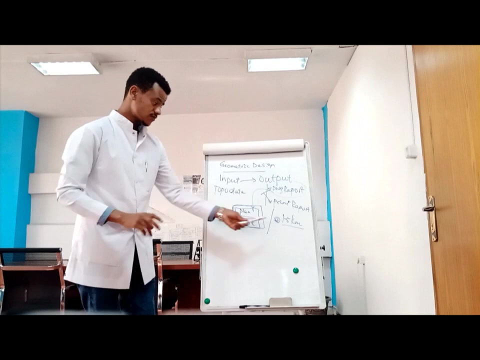 The distance between the two sides is 1.5 km. For example, if we are talking about 10 km, we can say that the distance is 1 km. If we are talking about 150 km, we can say that the distance is 1.5 km. 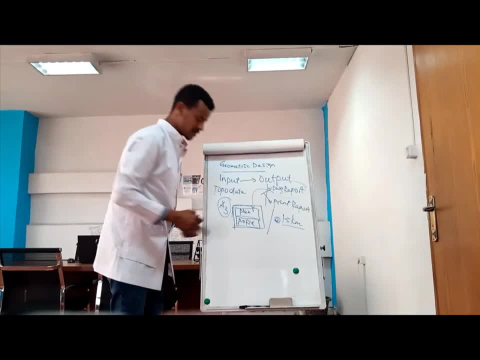 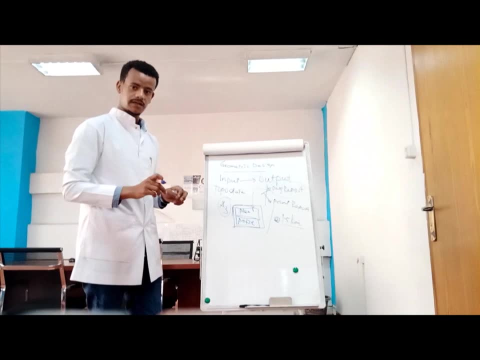 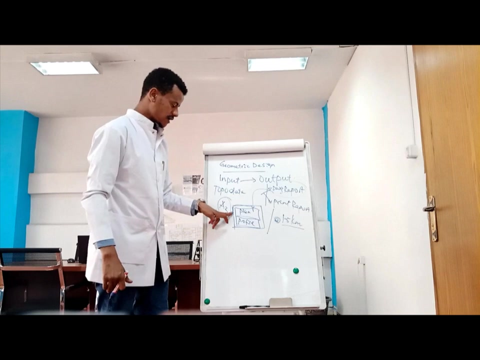 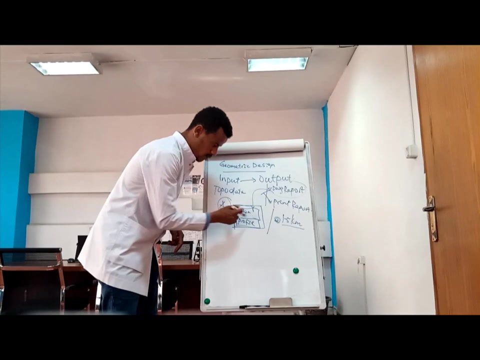 If we are talking about 150 km, we can say that the distance is 1 km. Therefore, I tried to be as realistic as possible When I had to activate the system. it did not be a detailed understanding. I also tried to test the processes in this way. 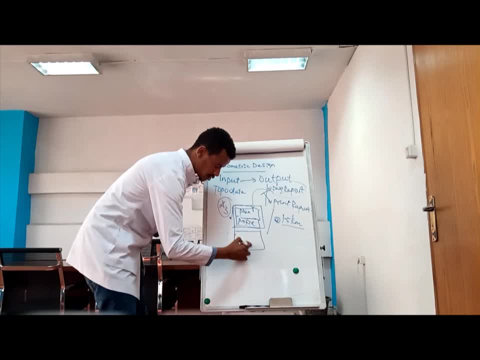 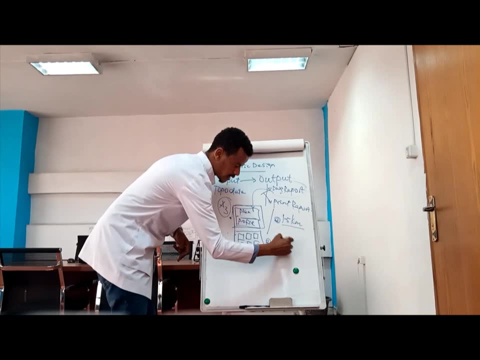 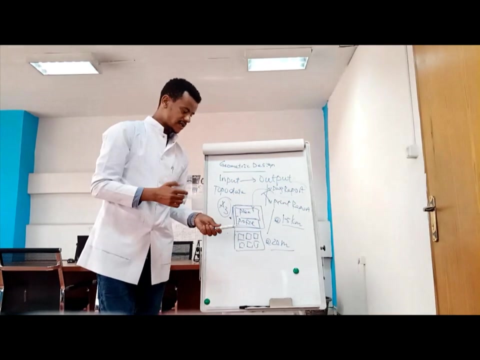 I have dealt with the cross-section also. When I held the machine and when the ml basket I had otraized the mat, it broke down. Here we have 20 meters. If we draw a cross-section within 20 meters, the report will be in the drawing. 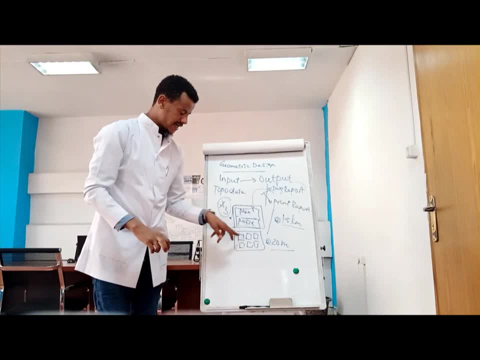 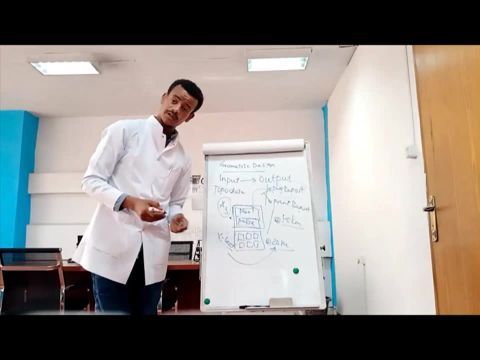 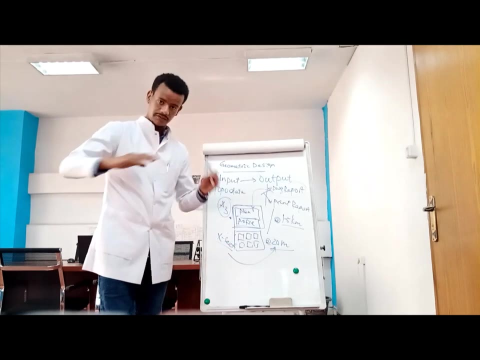 This is the third measure. In the drawing we draw a cross-section within 20 meters. When we draw a cross-section, the paper is not cut. The paper is cut When we draw a cross-section. we put a line in between the paper. 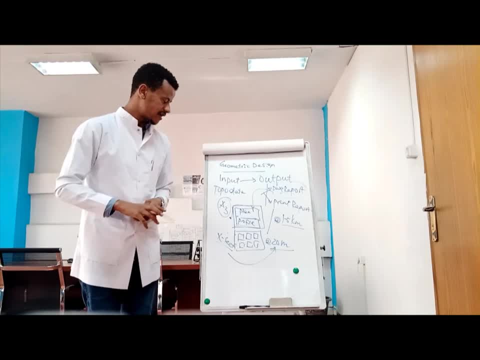 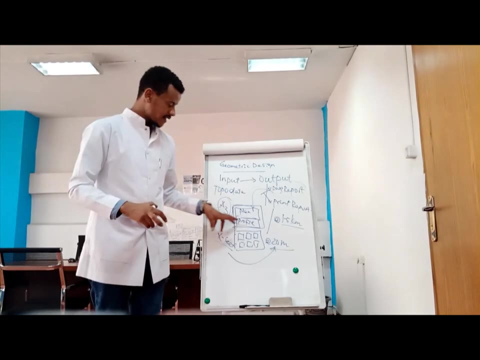 So we divide the paper and draw a cross-section. This is how we draw a cross-section. In this way, when you draw a cross-section, it does not take place. This is the same. The plan profile is the same as the previous one. the grid is the same as the previous one. 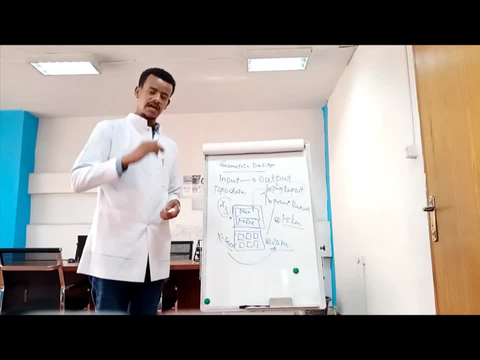 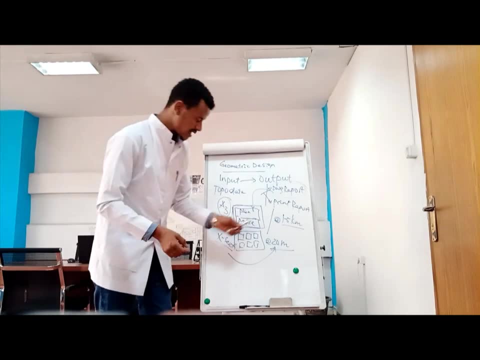 the control is the same, the plan profile is horizontal, the vertical curve is the same as the straight segment and the report is the same as the previous one. So this is how we can use the output in the drawing to make the drawing. 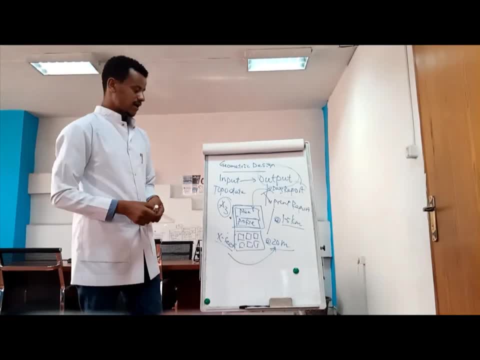 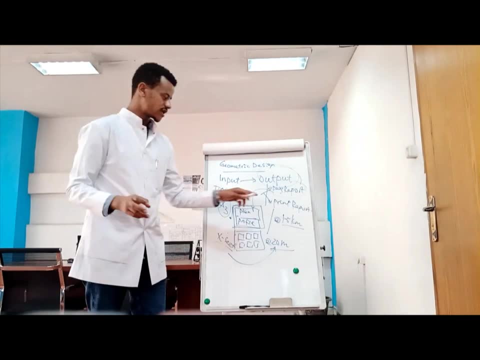 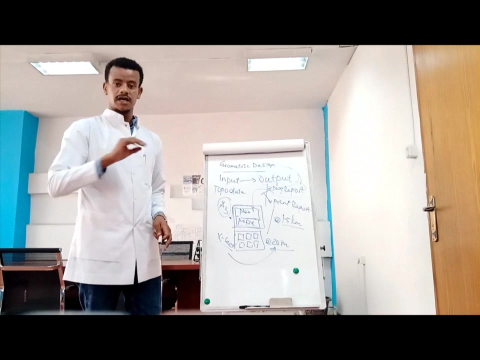 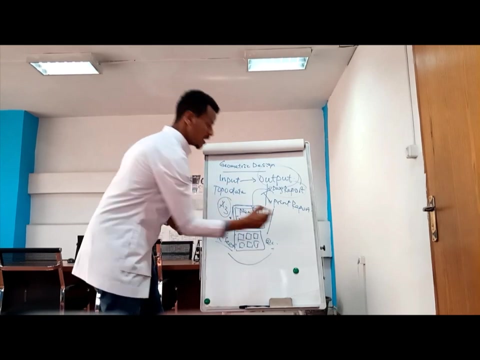 So this is how we can use the output in the drawing to make the drawing. Sometimes we don't use the print report, we use the volume report or we use the line graph. So we can use the drawing report to make the print report. 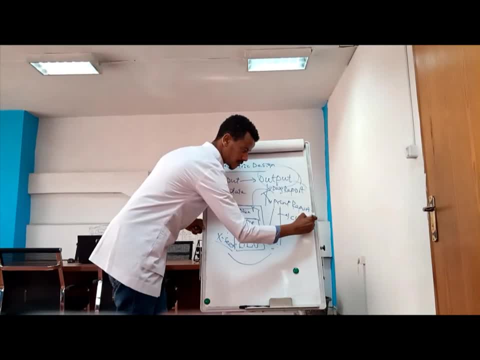 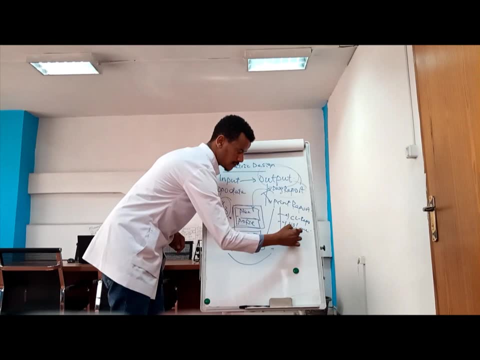 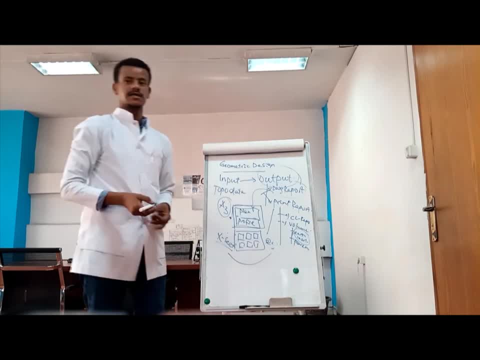 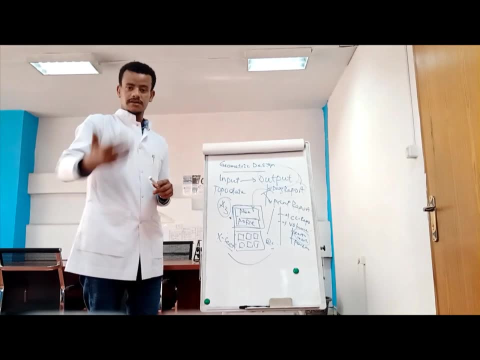 It Dakota non paper volume, So we report by volume In a regular geometrical way. if you decide to use a� Jennifer Logan s bombing speed mode, We will use the material to make a compaction. For example, the material of the base is about 7 cm. 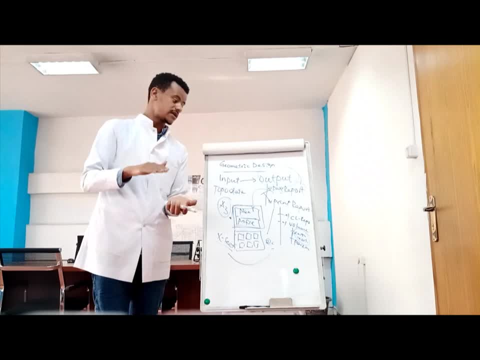 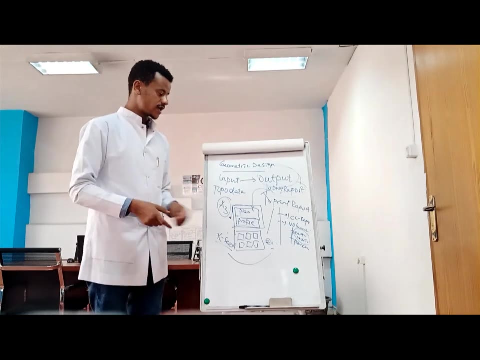 and we will make a compaction of 4 cm. Then we will use the material to make a shape of a millimetre. The shape of the material will be the same as the material of the base. We will use the material to make a shape of a millimetre. 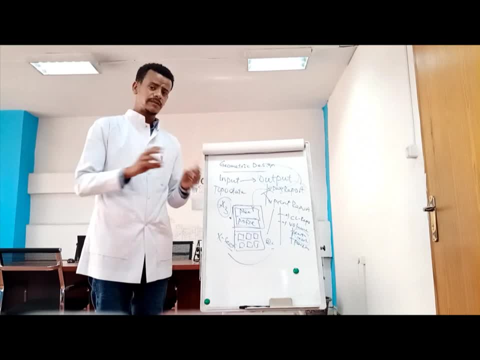 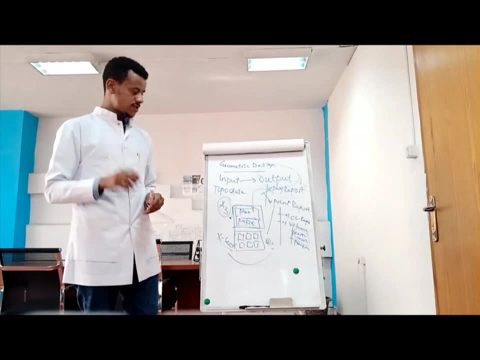 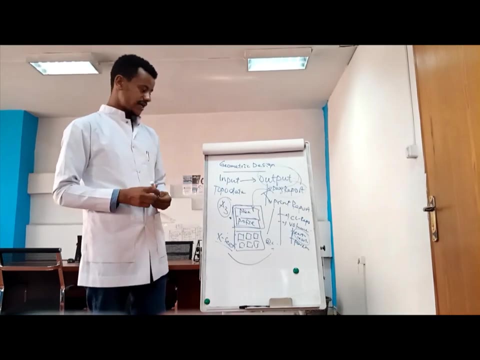 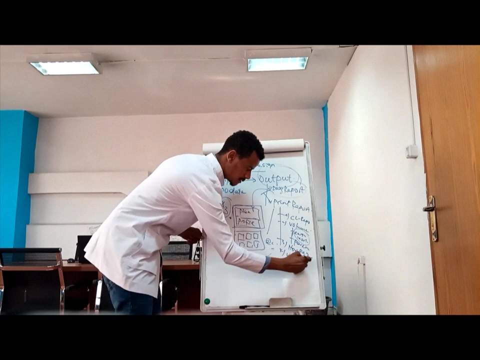 We will also use the volume of the material to make a shape of a millimetre. We will use the material to make a shape of a millimetre And we will also use the volume of the material. The first thing we will do is to make a vertical report. 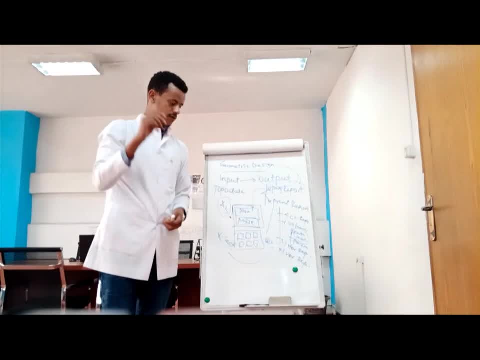 If the vertical report is not good, we will use the curve. If it is not good, we will use the curve. It's a straight segment. If you look at it from the side, you can see the curve details. The straight segment is the same. 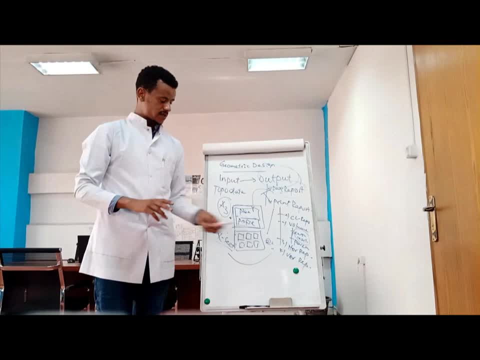 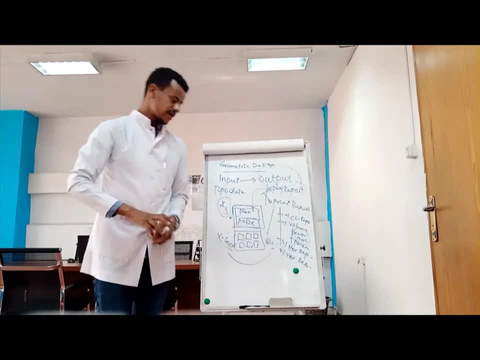 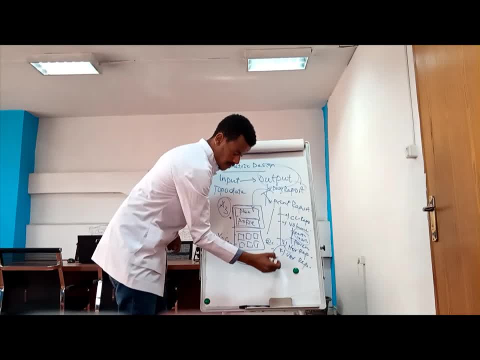 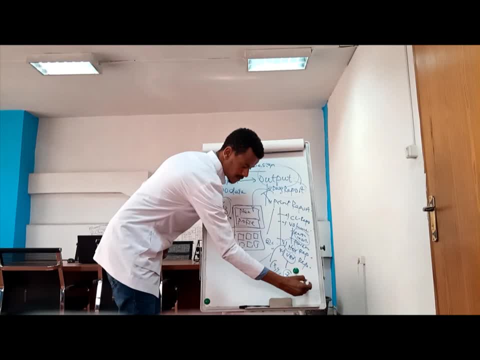 It's the same curve. This is the same curve. This is the same curve. The line is greater than b. I'm going to show you this curve again. This is a b curve. I can show you this curve again. You can understand this curve. 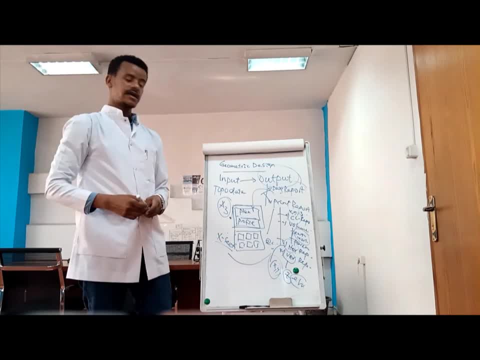 It's a line that looks Wilkman curve. This curve is at the natural center of the line. This curve has to do with movement of both planes. It's the same curve on both sides. It's called seают roster. It's the same curve on both sides. 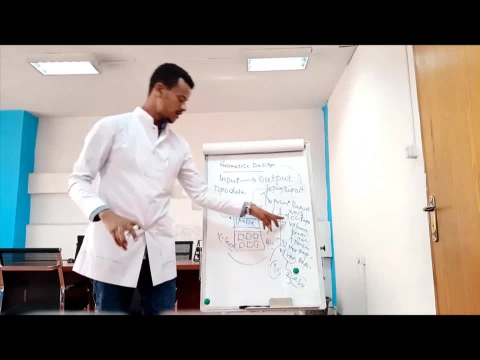 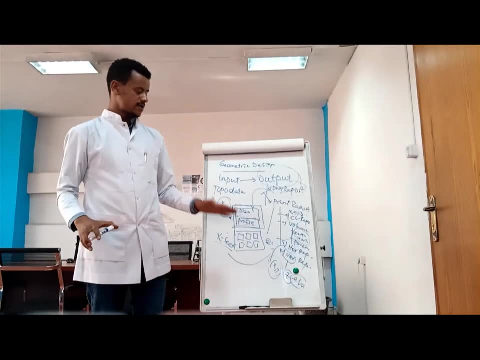 It's nothing like this curve. It's a crises form triangle design of the guys. I am going to show you how to make a vertical line with the help of a ruler. I am going to show you how to make a vertical line with the help of a ruler. 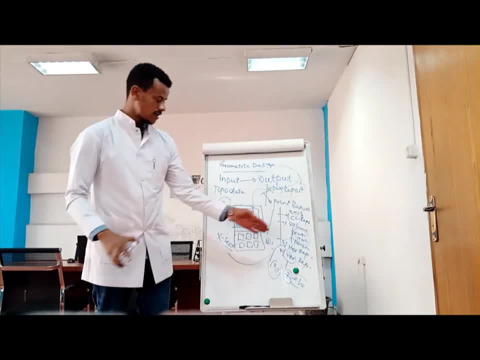 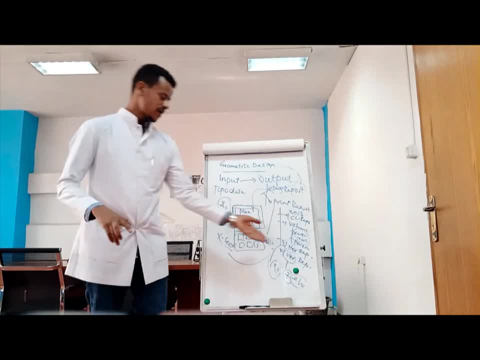 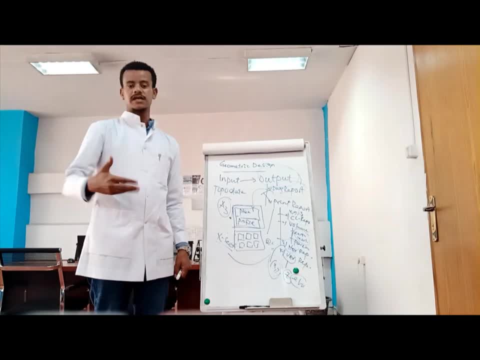 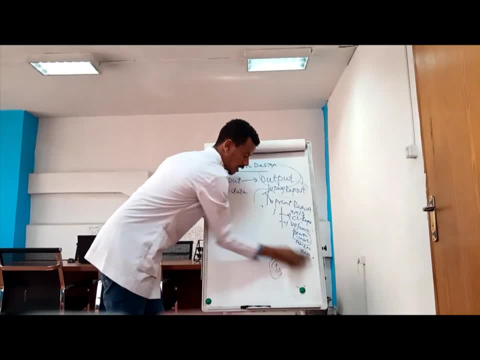 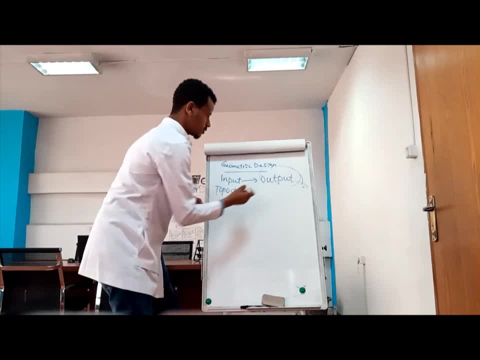 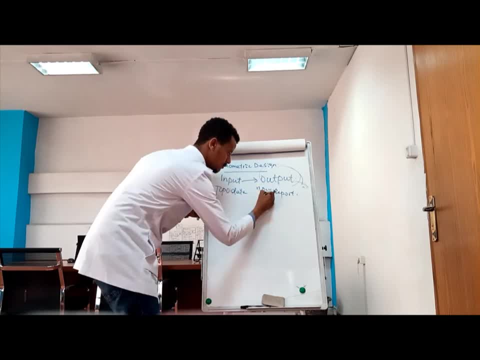 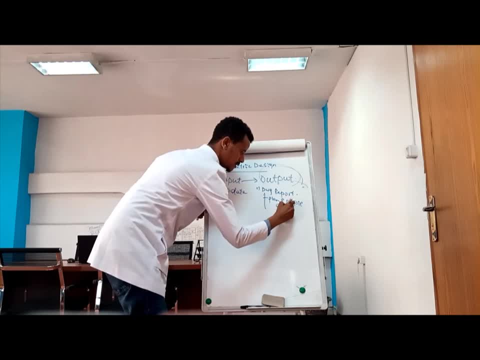 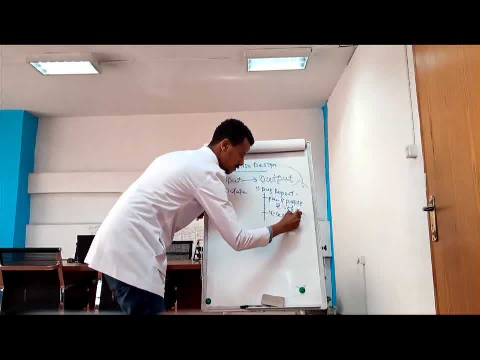 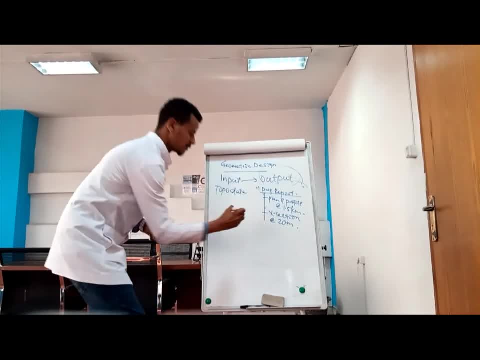 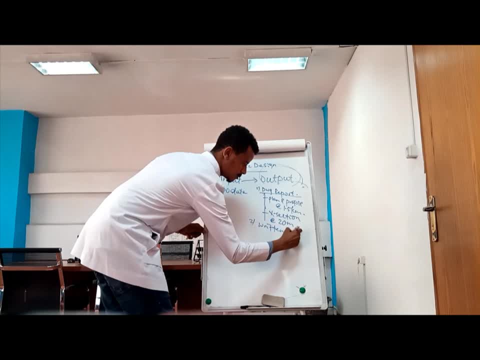 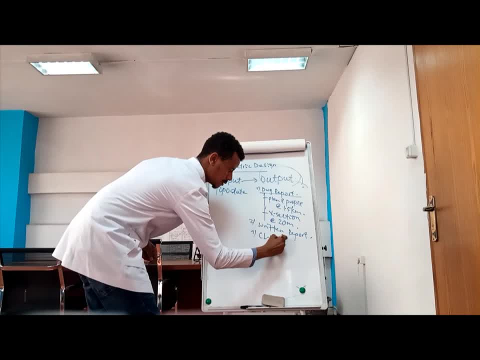 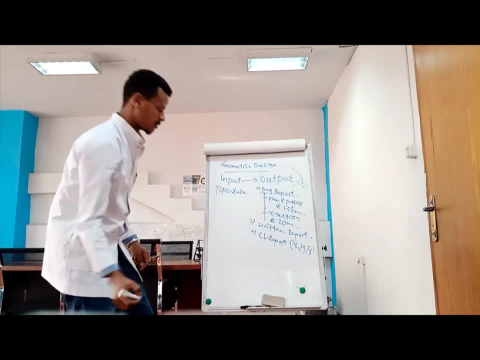 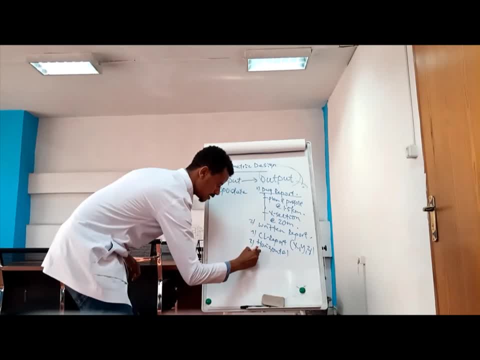 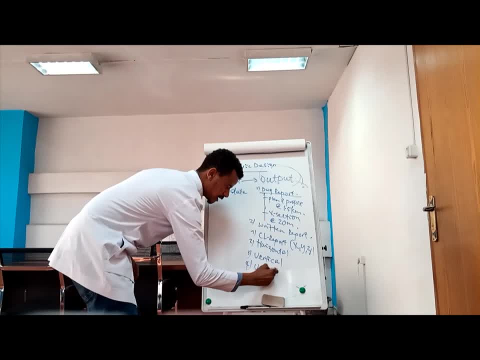 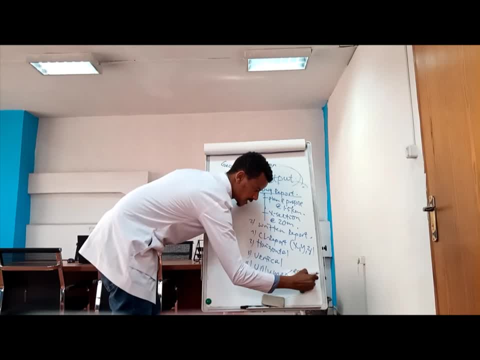 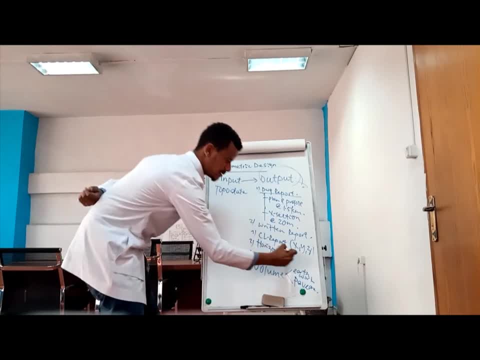 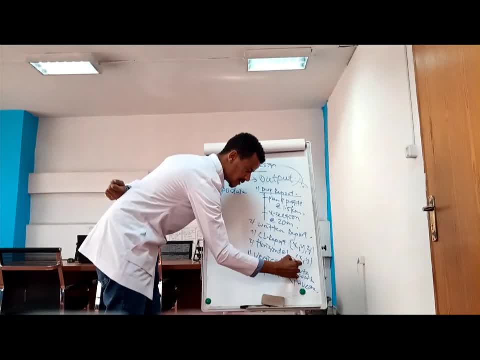 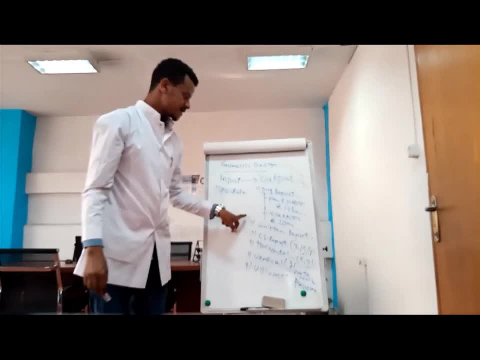 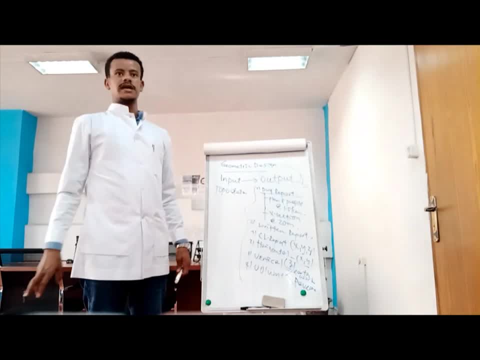 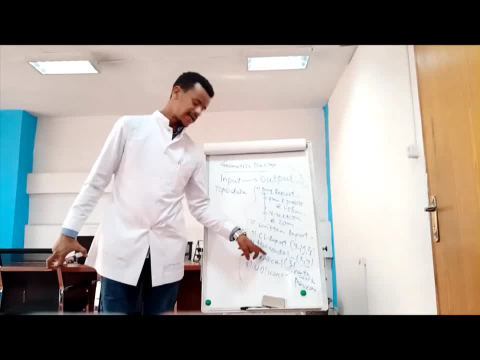 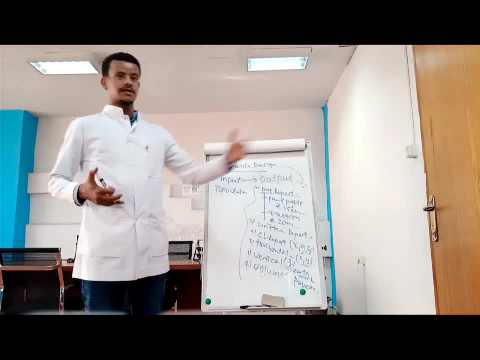 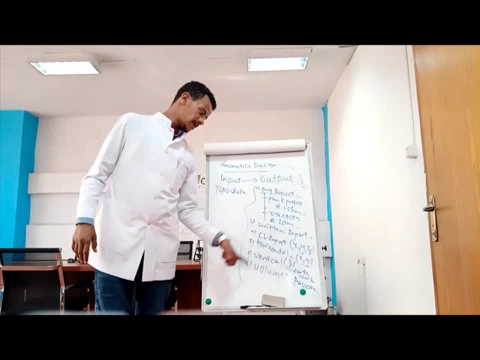 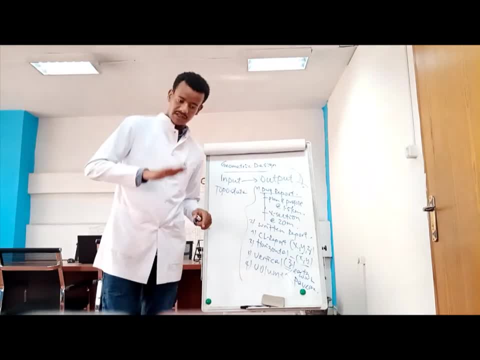 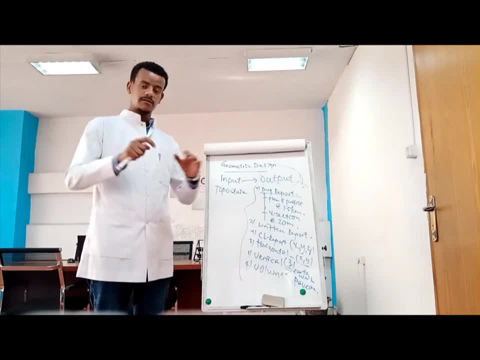 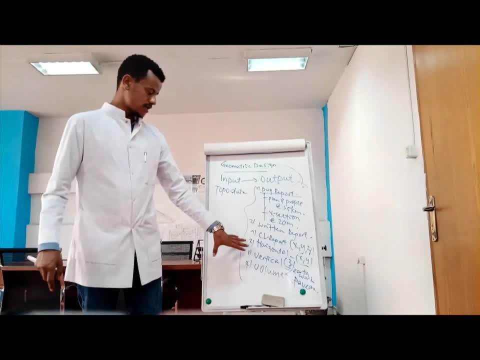 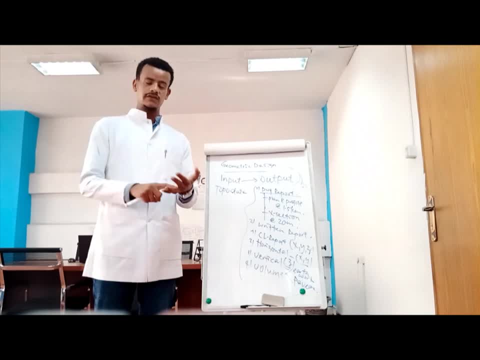 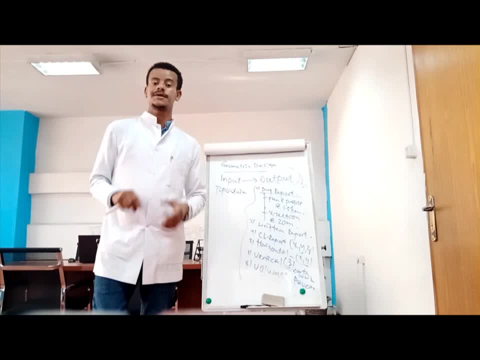 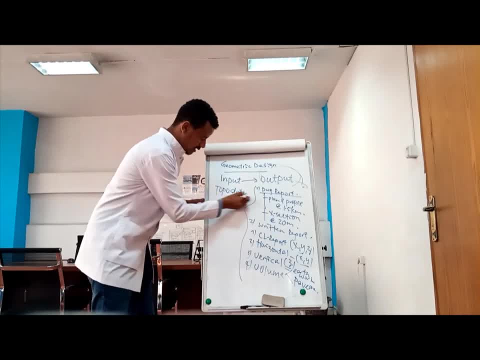 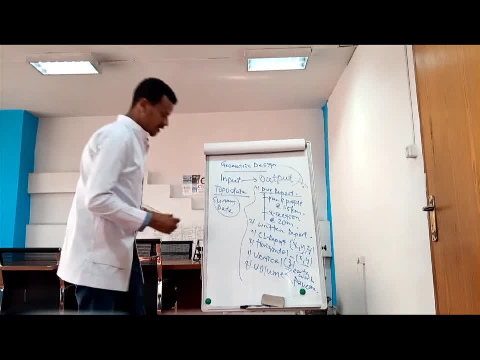 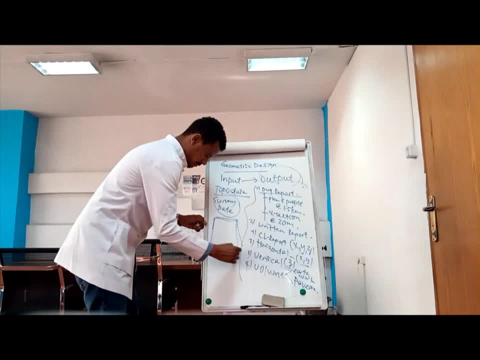 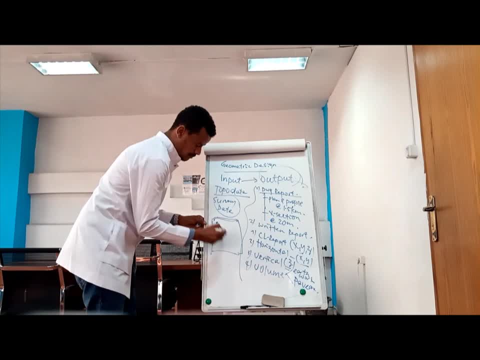 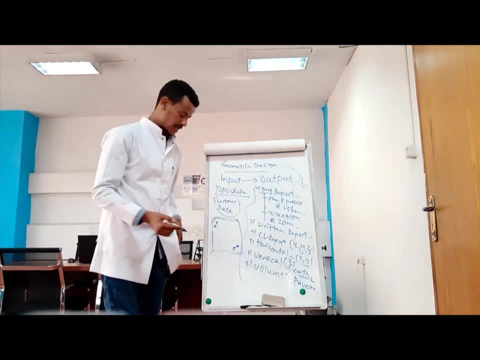 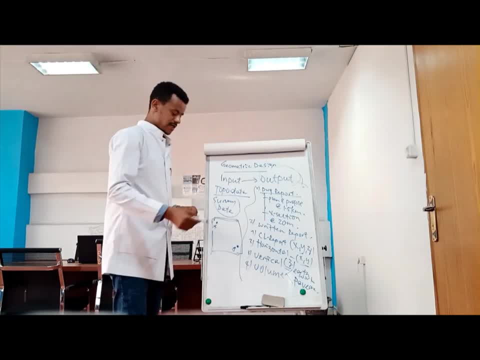 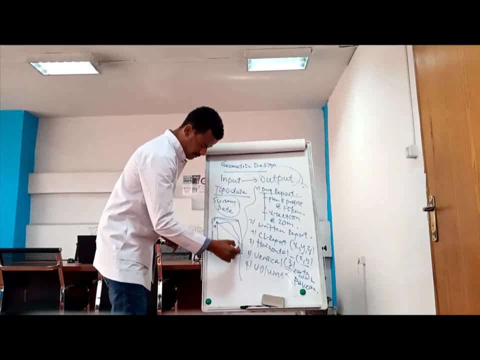 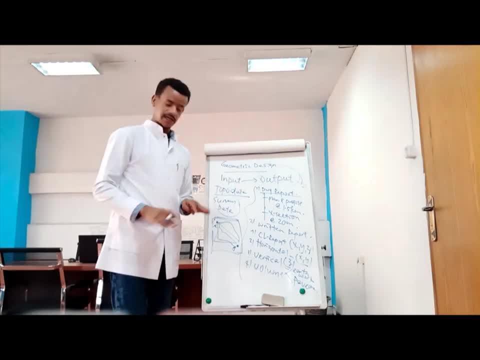 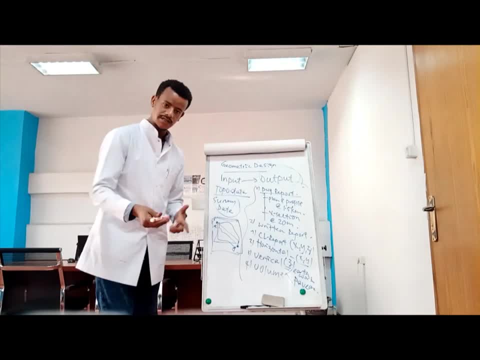 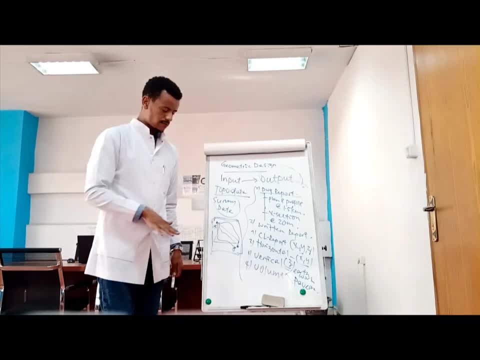 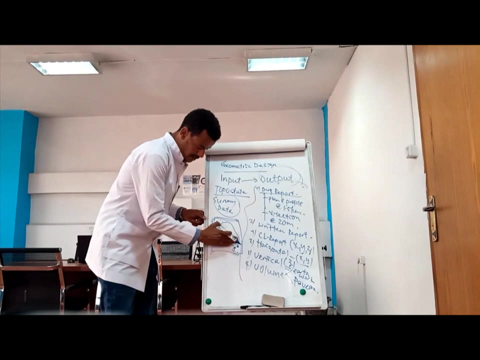 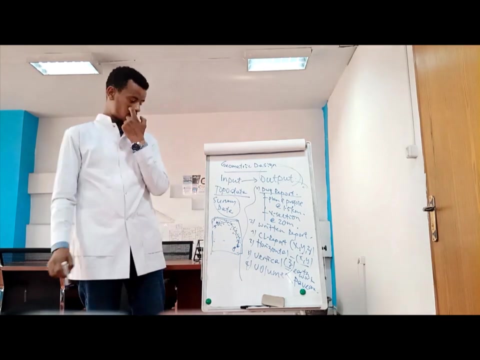 I am going to show you how to make a vertical line with the help of a ruler. I am going to show you how to make a vertical line with the help of a ruler. Soon Meta Core Topo Data Is called Natural Merit. 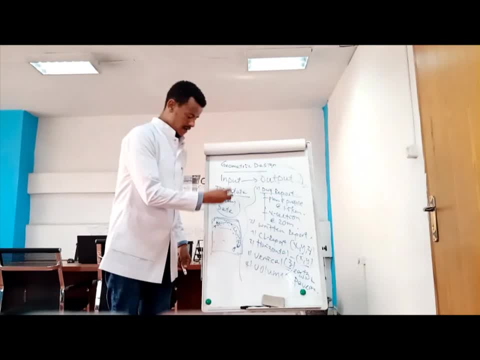 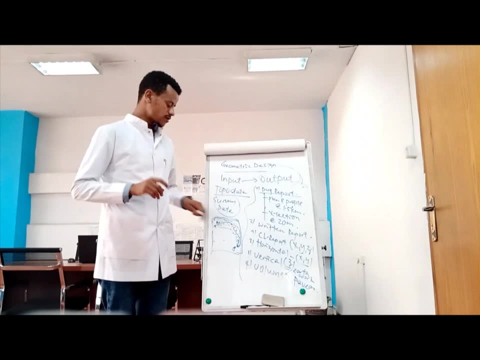 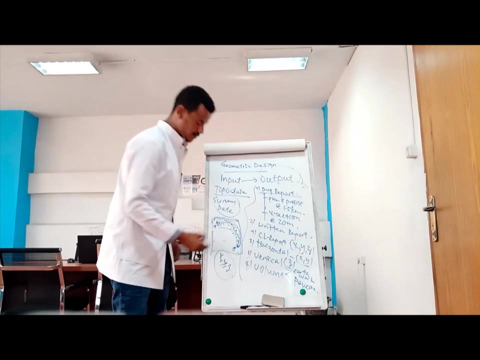 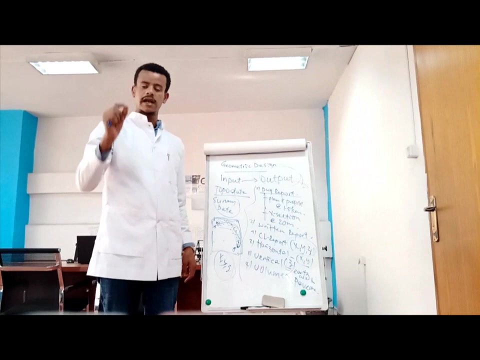 The Natural Merit Is a physical, Natural, XYZ Coordinate. Merit Is a physical Before the design, It's an XYZ Coordinate, This XYZ Coordinate. Finally, This is the final version of the smooth horizontal and vertical fit of the smooth. 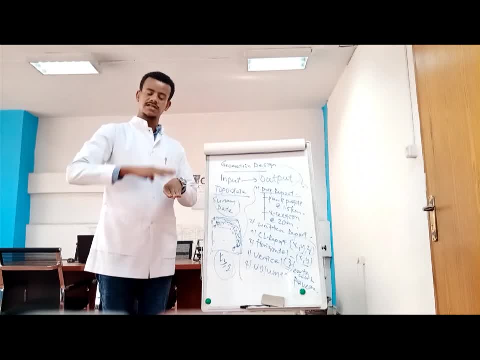 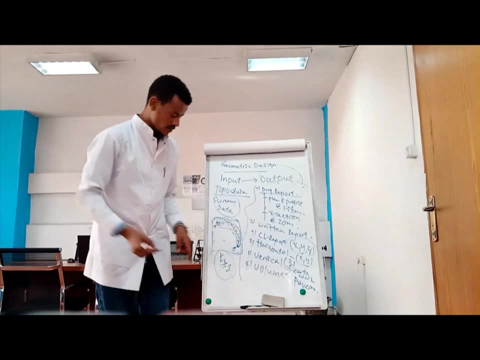 The corners are definitely graded. The design of the smooth is limited by the mass of the machine and the mass of the machine itself. The design is graded. Now let's look at the colors. The color of the random is zebra and the color of the natural is red. 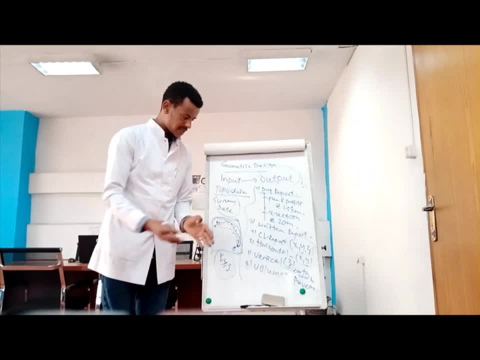 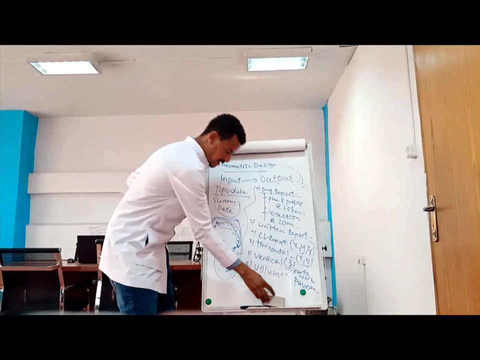 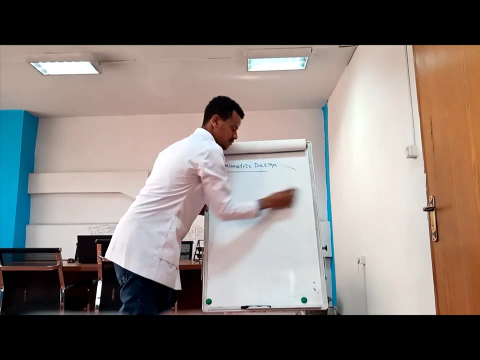 The black color is a combination of the colors of the smooth horizontal and horizontal fit. The colors are red and blue. In this case, the snow is red. The color of the smooth is green and blue. The colors of the smooth and red are yellow. 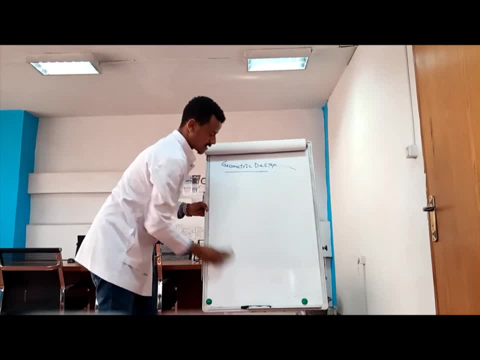 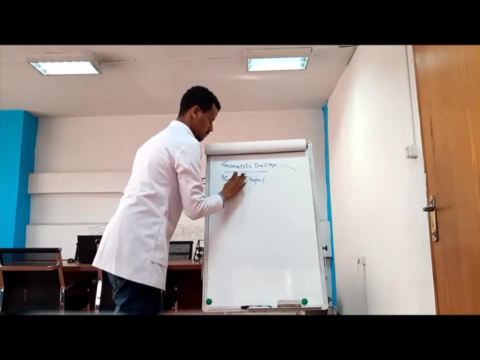 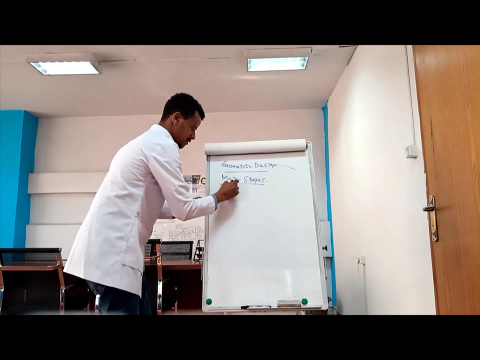 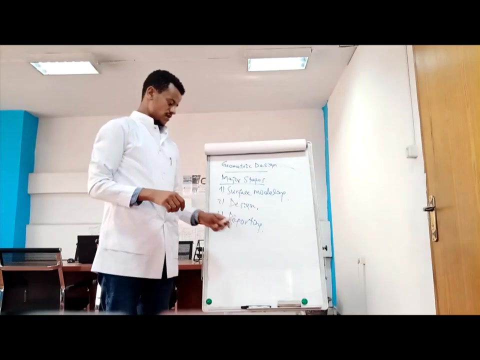 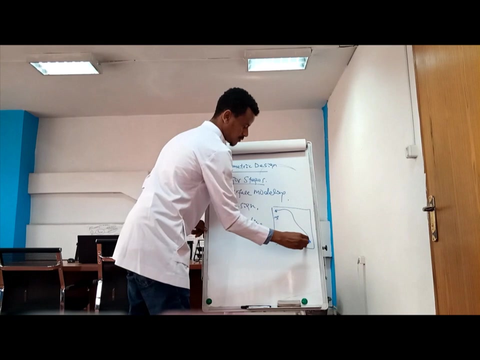 The colors of the smooth are orange and orange. The colors are brown and purple. The colors are blue and blue. These colors are purple. I will show you the major stage of work: surface modeling: design source and report For surface modeling, for example, CTN and CTB. I am going to show you how to create a topo data. 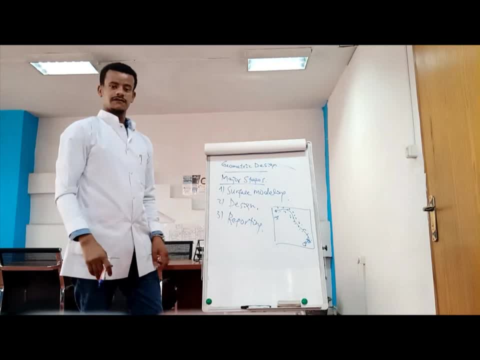 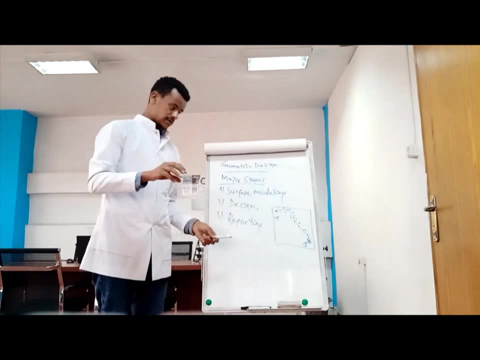 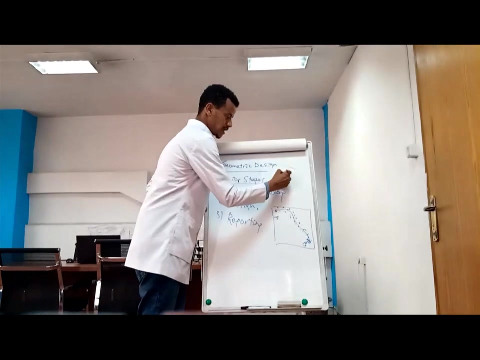 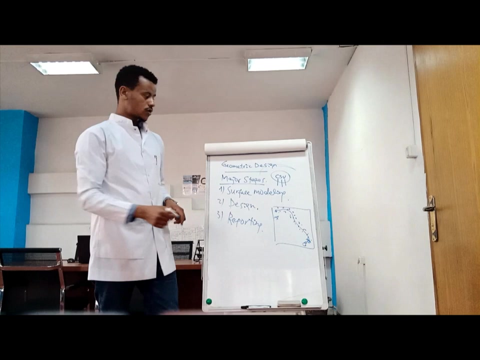 I am going to show you how to create a topo data with the original topo data. The program is a mirror format. The format is basically CSV format. CSV format means that all the columns are separated. The format is exactly the same as the Excel format. 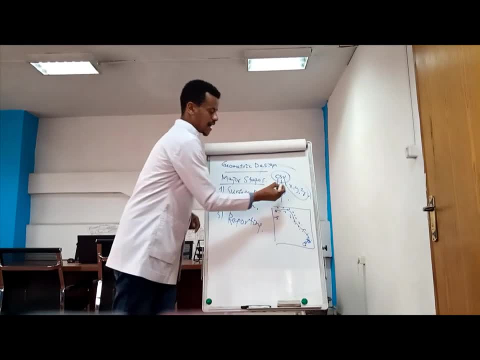 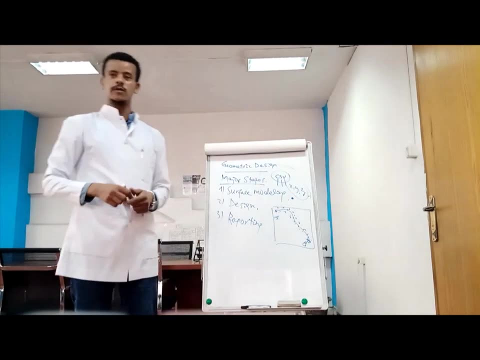 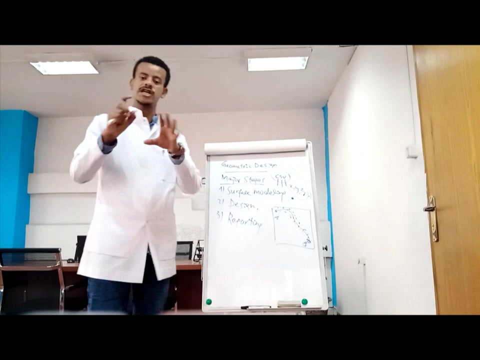 I'm going to show you the coordinators in subgroups such as X, Y and Z At the end. the data is divided into three main groups. In this case, the training includes professional data, social data and training. I am going to show you some of the data that is actually in the training. 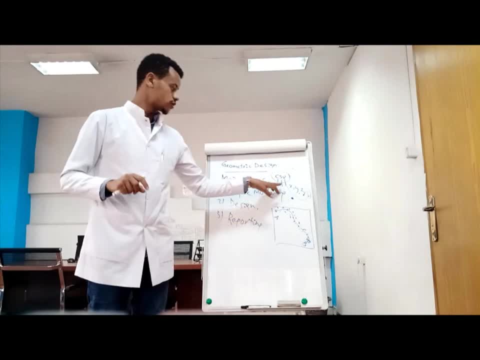 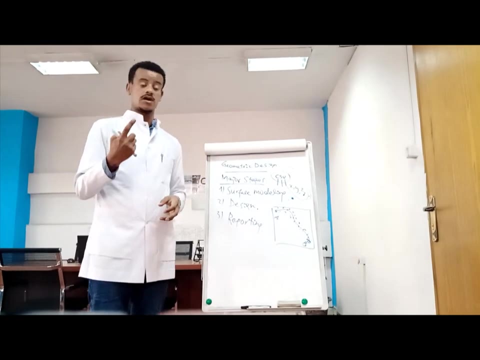 The X, Y and Z coordinates are the source coordinates, but they are telling you about one point. So in the CSV format the data has a different role. The source coordinates are the one point and the separated values are the definitions. 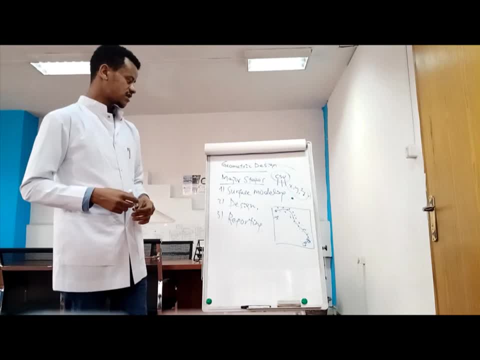 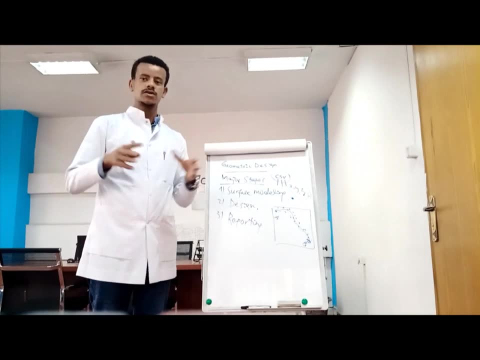 This format is very important in the program. So surface modeling is the main function And we can use it to make some kind of a square, For example the shape of the square, the height, the height of the square, the width of the square, the smoothness of the square, etc. 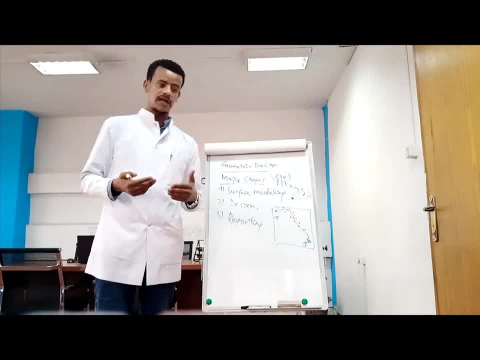 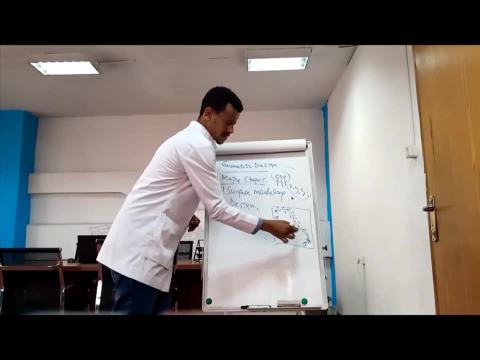 We can make some kind of a square And then the coordinates can be used. to give you the coordinates. If you use a coordinate, then you can get 100% of the data, which is ideal, But you need to be careful. 17., 18., 19., 20., 21., 22., 23., 24., 25., 26., 27., 28., 29., 30., 31., 32., 34.. 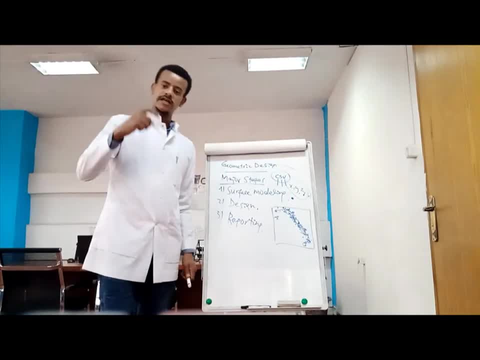 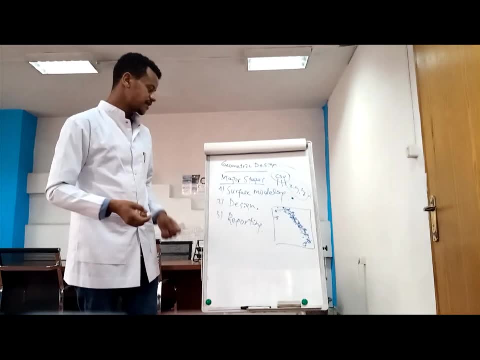 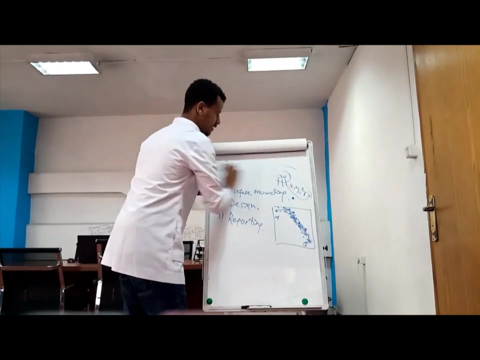 35., 36., 37., 38., 39., 40., 41., 41., 43., 44., 44.. So surface modeling is a special stage. surface modeling is what I am going to talk about in this video. 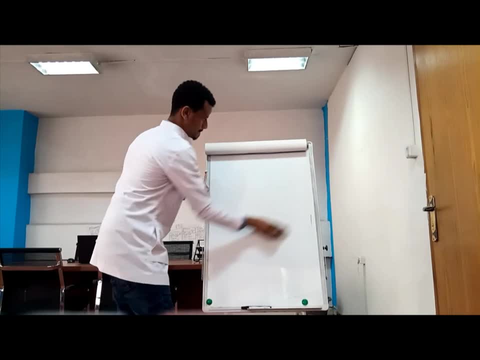 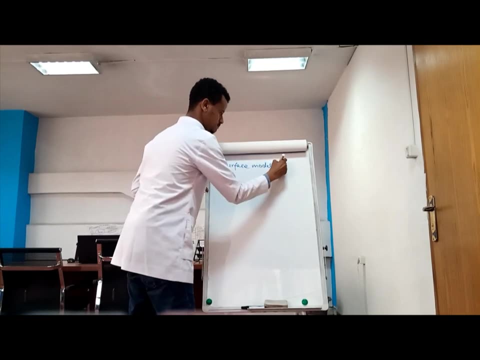 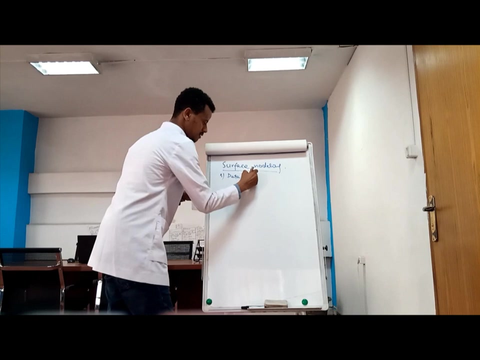 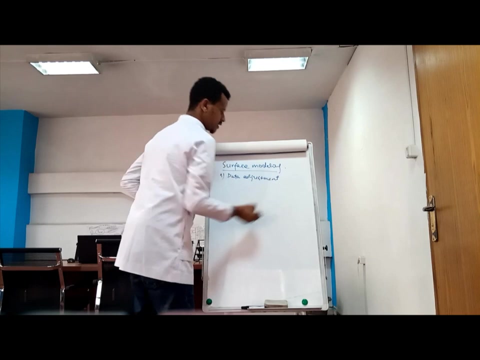 Surface modeling is a service. surface modeling is a service. surface modeling is a service. The first thing you need to do is data adjustment. The first thing you need to do is data adjustment. For data adjustment, you need to start with the topo data, the data from the server. 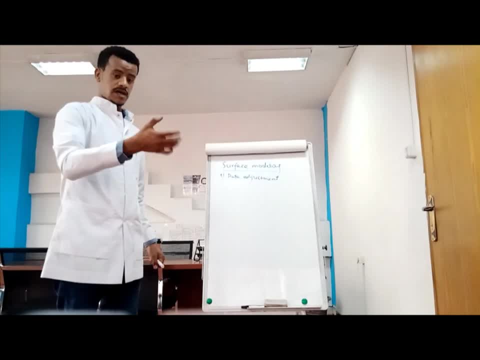 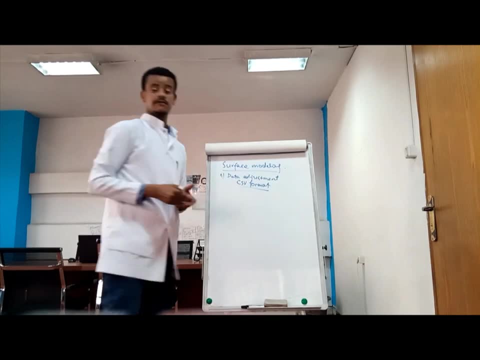 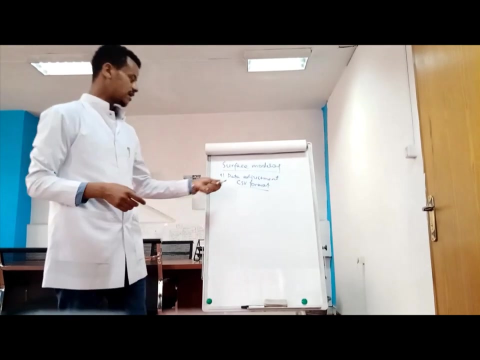 For the program. you need to go directly to the input meter. I will show you how to do it. First, you need to introduce the CSV format. The CSV format is a comma-separated-value format. You need to import the program. The format is just a comma-separated-value format. 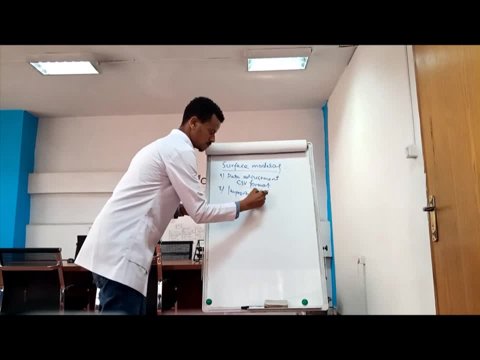 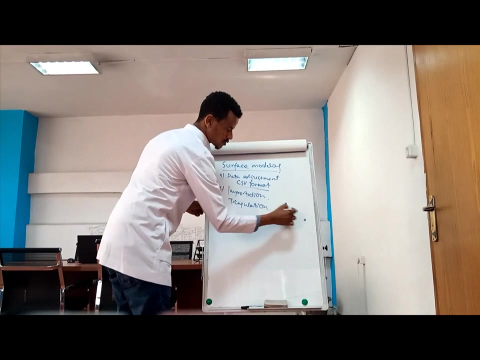 In this case, the format is importation. The import is not important, it is import In source. you need to import triangulation. Triangulation is a major stage When you want to run an image in source. you want to take the source point to the area of the image. 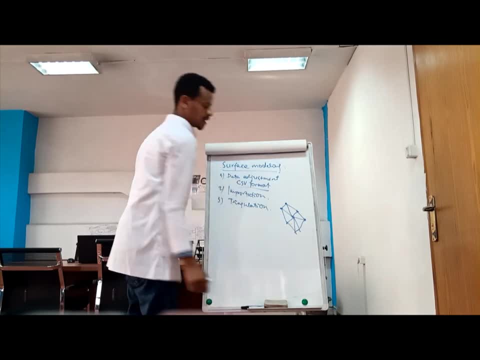 When you need to perform a Jangulation, you can go to the source point, to the area of the image. In the previous video we saw how to do triangulation, So triangulation- as the name indicates, it is triangular formation. 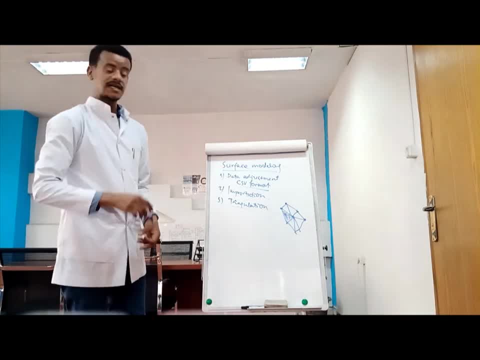 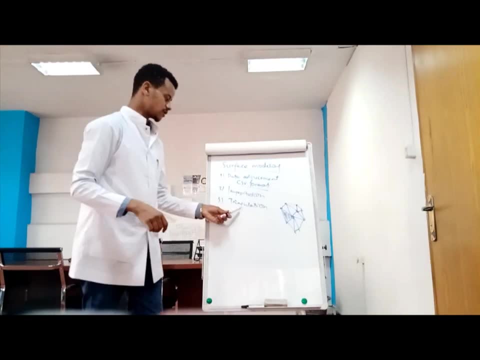 We have a triangle, a multiple of triangles. We want to have a triangle that is not at one point but at another point. We want to have a triangle that is not at one point but at another point. This stage is the key for surface creation. 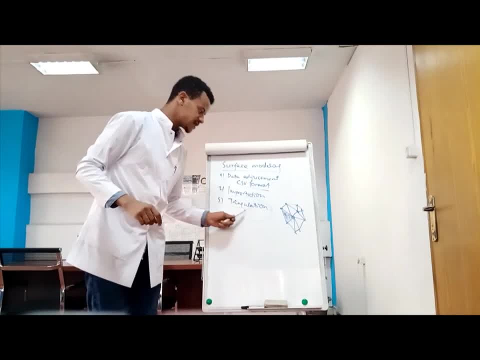 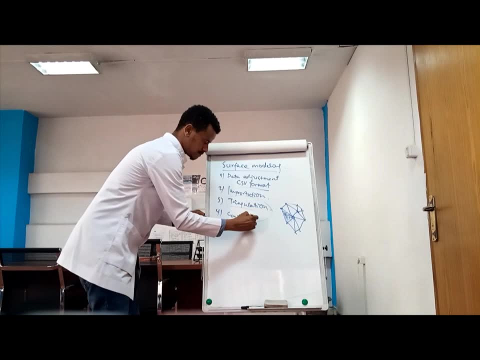 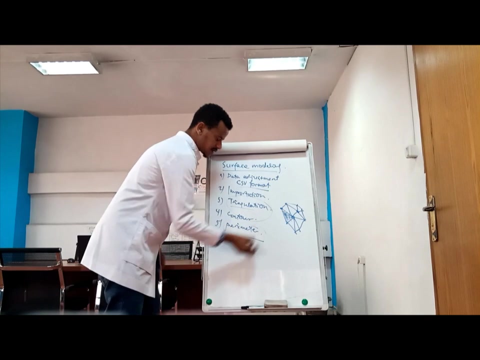 Basically, we call this stage triangulation. We will be using this stage to make a straight line. So triangulation is the step to make a contour. The next step is parameter. We will be using this parameter Now. if we look at the line, we will see that it is 1 meter wide and 1 meter deep. 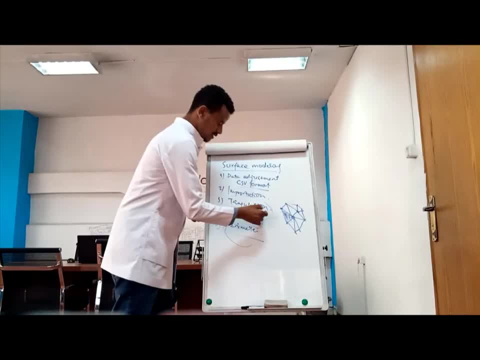 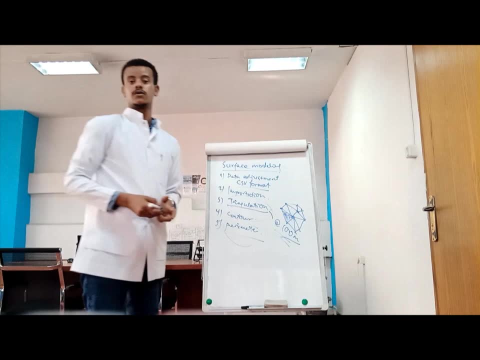 Basically, the line is in a straight line, So the triangulation is at a straight line and the point is at 100 meters. If we take the conventional method of triangulation, 100 meters by 100 meters, we have 100 meters. 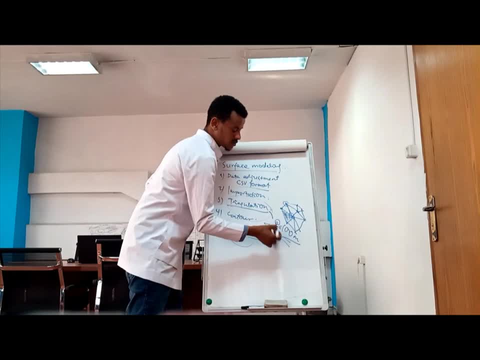 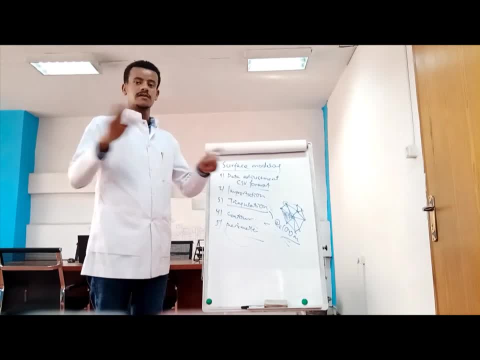 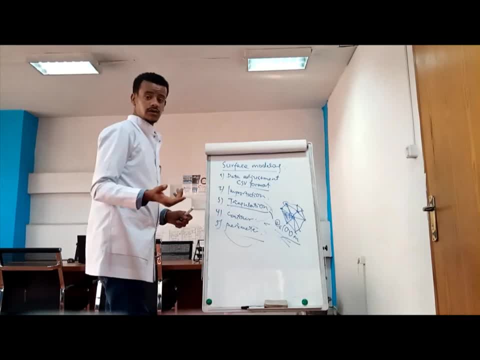 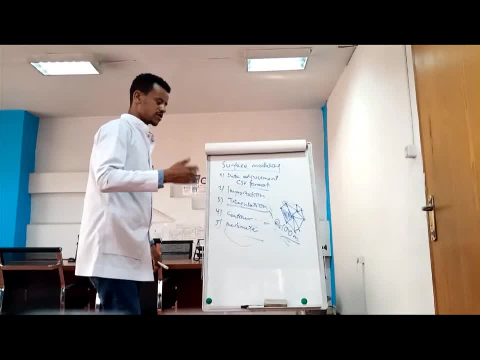 At this point, we can see that there is a lot of noise. We can see that there is a lot of noise. At this point, we can see that there is a lot of noise. At this point, we can see that there is a lot of noise. 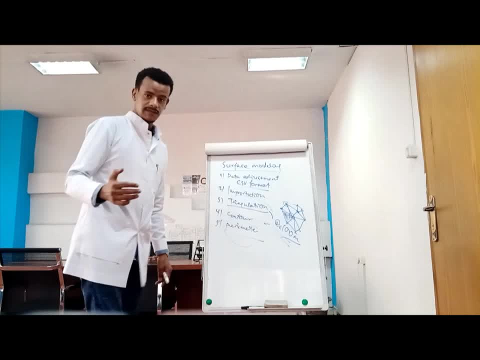 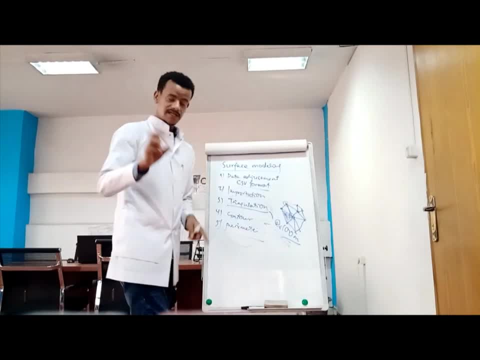 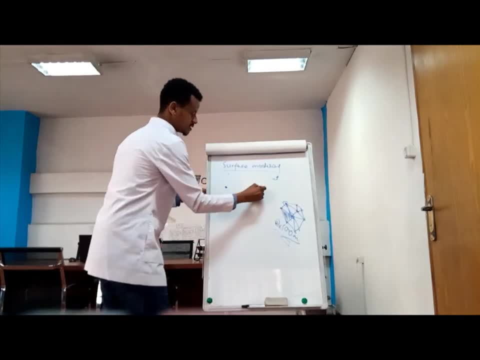 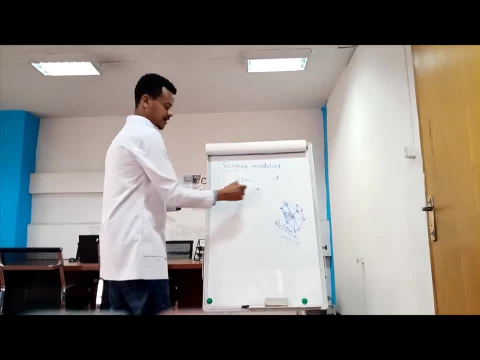 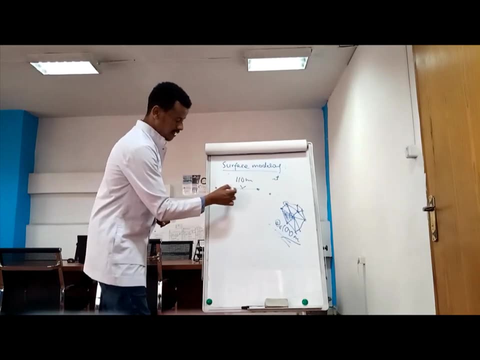 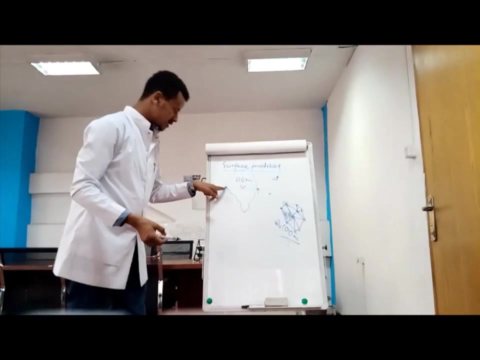 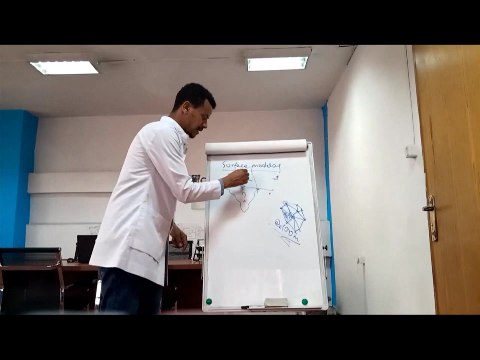 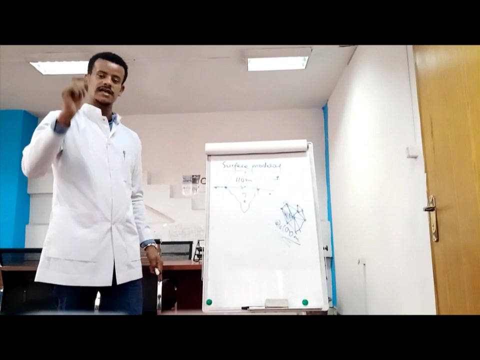 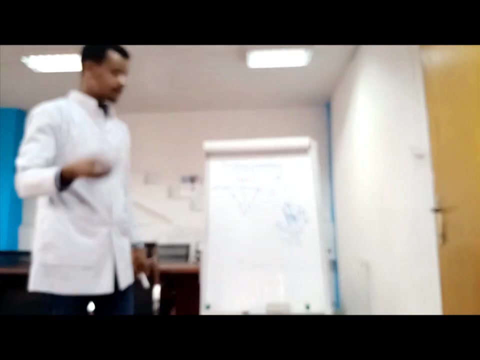 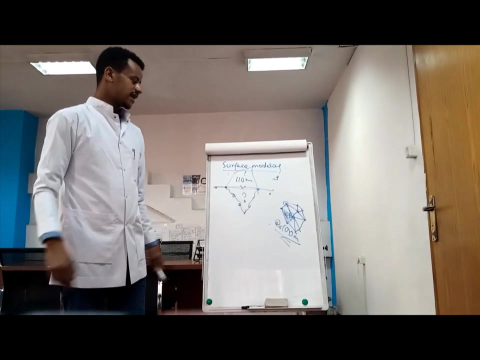 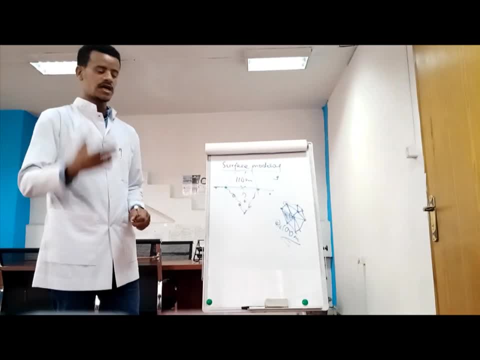 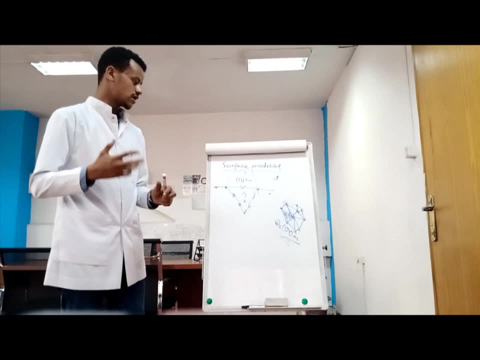 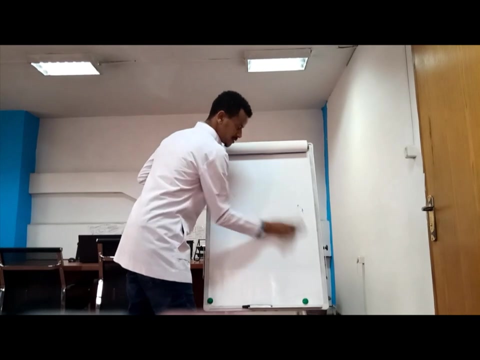 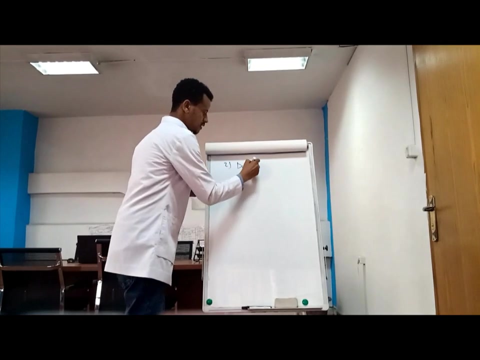 In our work. we design our kreatme for 3-conditioned and made this concept about surface boolean, which is an artificial simulation platform. Every design is何 We have to write like a landscape. All you need is a plan, a some precise and söyled plan, and basket about all these variables and package. 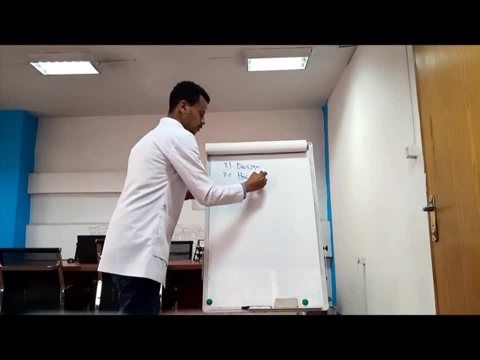 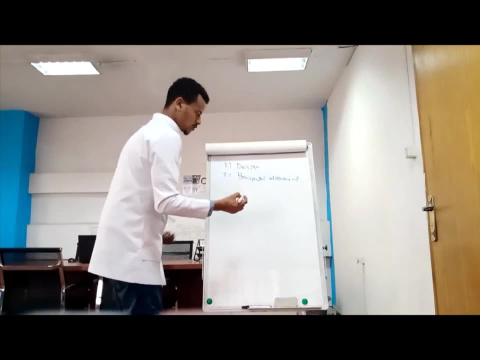 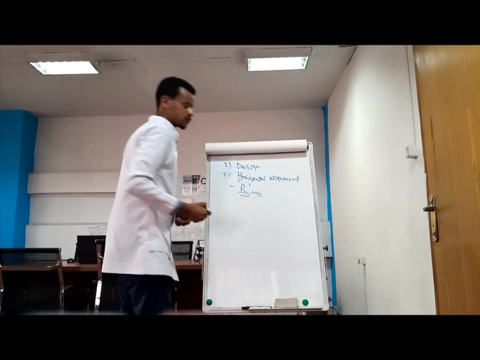 What do we do with this Kingdom? Do like us. This is the horizontal alignment. In the horizontal alignment, we can see that the area of the sun is different from the area of the moon. The design of the moon is similar to that of Arminian. 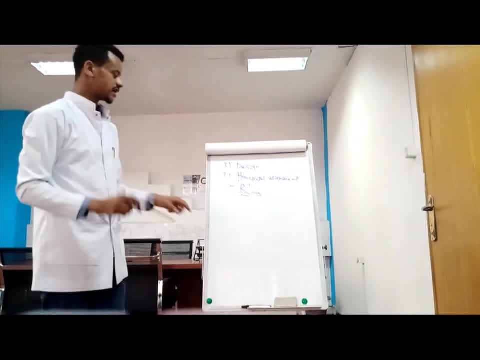 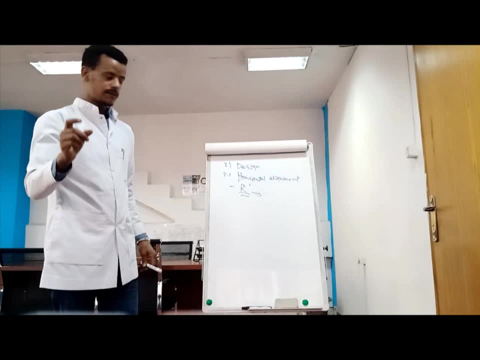 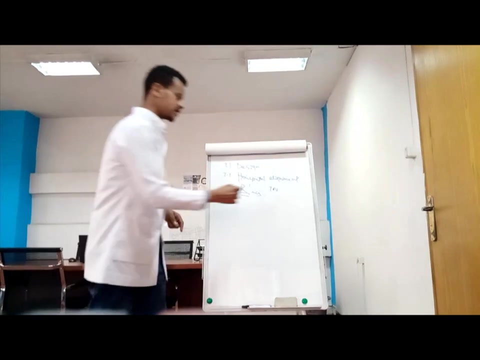 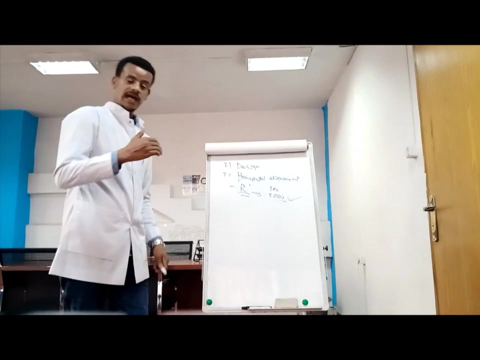 The design of the moon is similar to that of Arminian, because the radius of the moon is the same as the radius of the sun, But when the moon is drawing the twints, like you can see here, it is longer than the sea top of the moon. 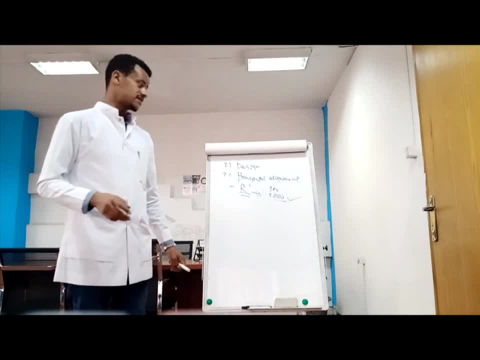 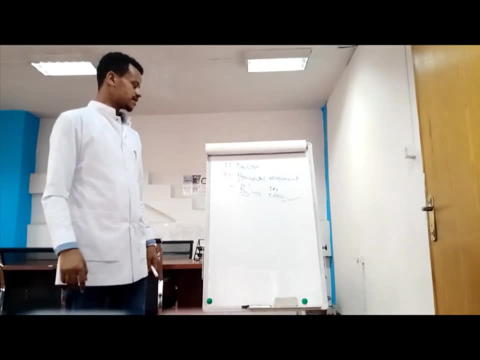 And the size of the sun over there is different by the time the moon is drawn. Theивают is cool. I think Yes. The next step is to reduce the weight of the car. The next step is to reduce the weight of the car. 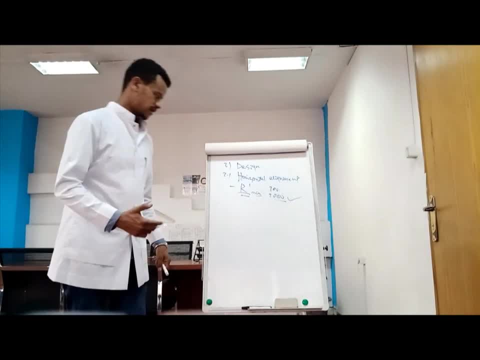 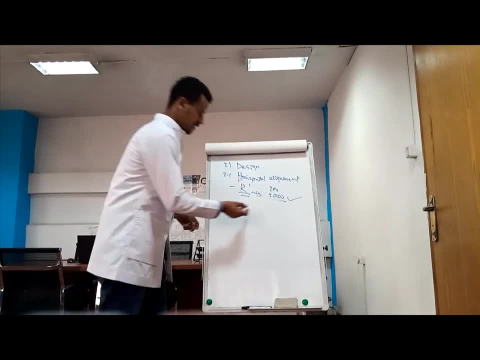